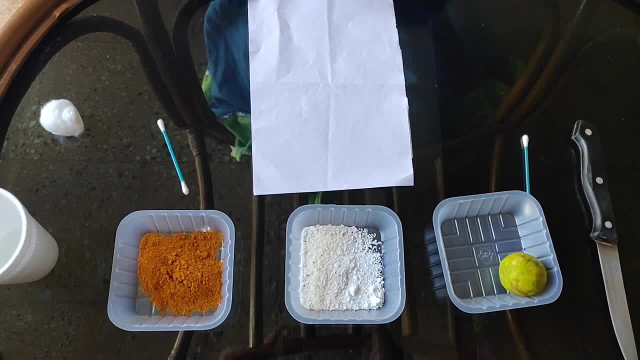 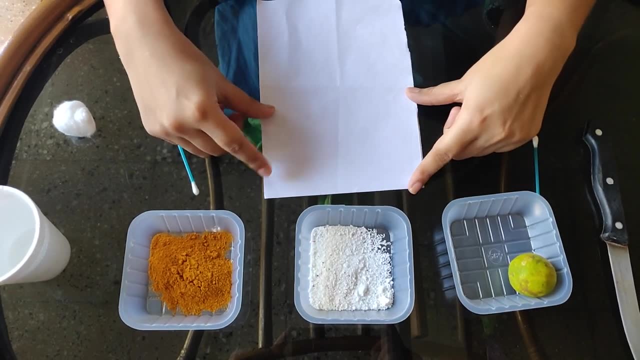 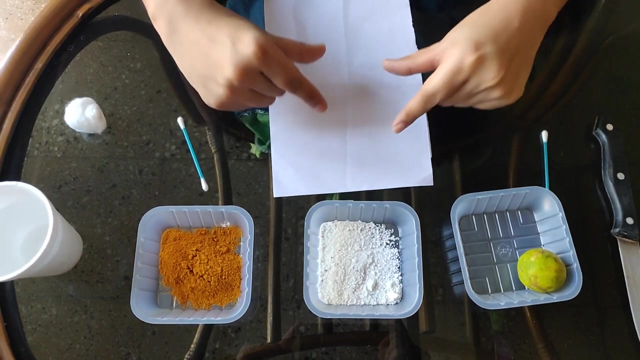 Today I will perform one activity for you where I will tell you how we test from turmeric indicator. Okay, so I will prepare one turmeric card for you all and you can check how what I have done and how I have used this turmeric card to check whether the substance is acidic or basic. 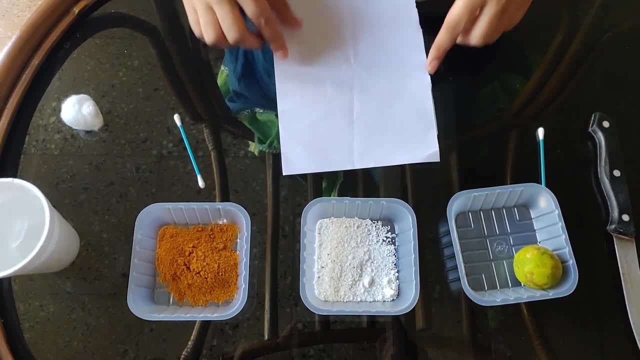 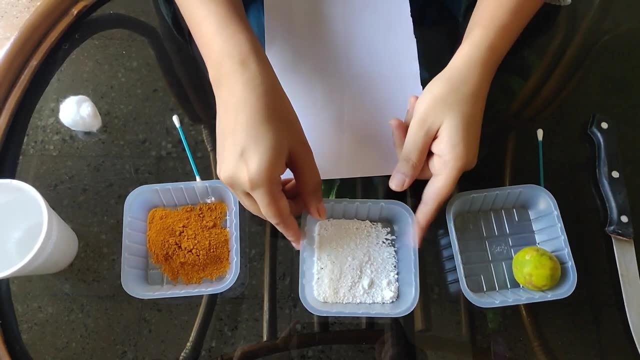 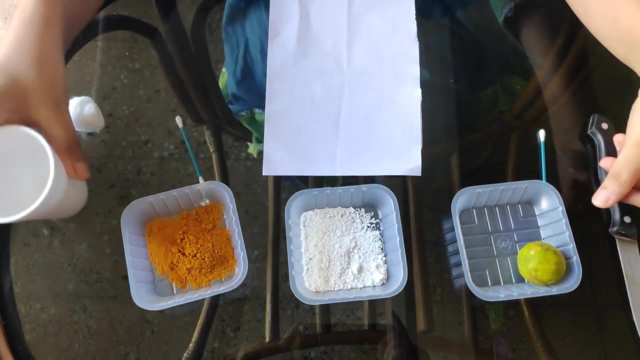 Okay, so now the materials that I have with me to prepare this activity is you can see this is turmeric powder, you can see this is detergent, okay, and this is a lemon and here in this glass there is a water. So first what I will do, I will make a turmeric paste. 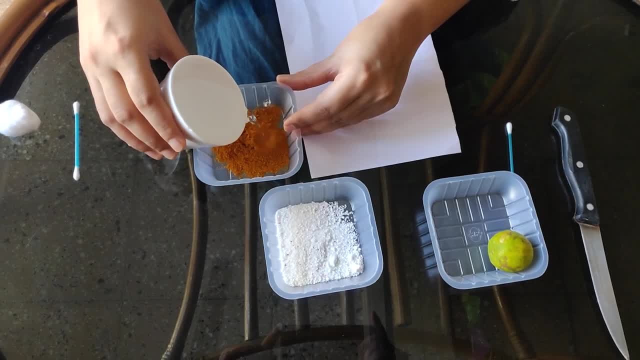 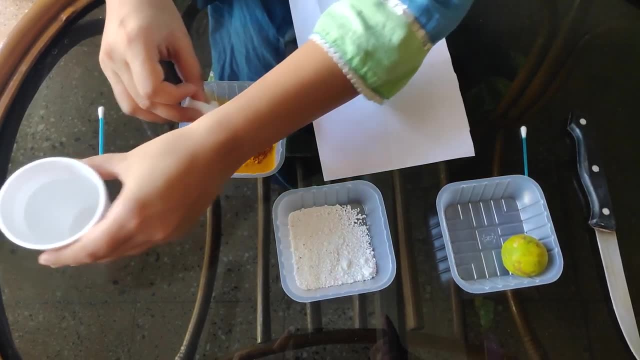 I will add few drops of water. I will add few drops of water to turmeric. I will prepare a turmeric paste. Now, this is my turmeric paste. 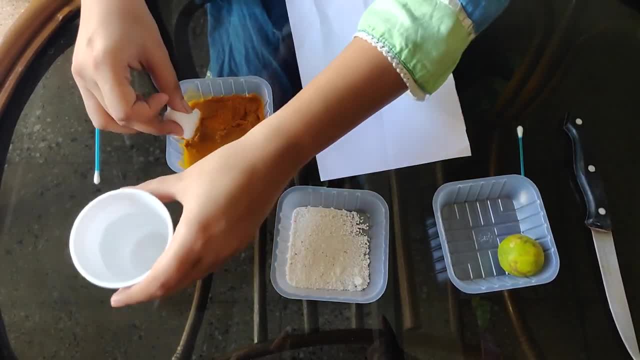 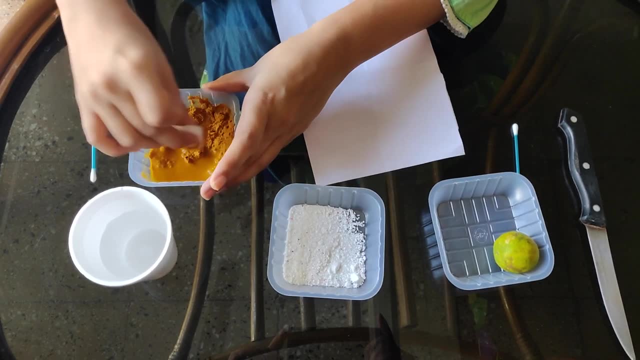 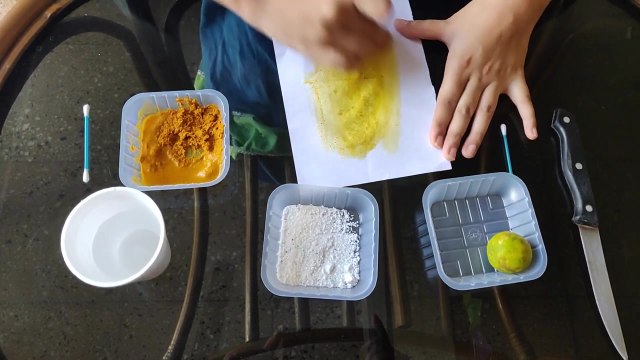 This is my turmeric paste that I have prepared by adding few drops of water. Now this turmeric paste I will apply with the help of cotton to this paper but you can use paintbrush also. Okay, anything you can use either you can use paintbrush or you can use cotton whatever the things you people have at home so you can do that. 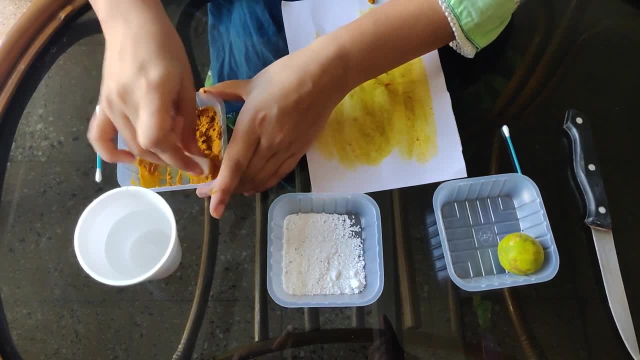 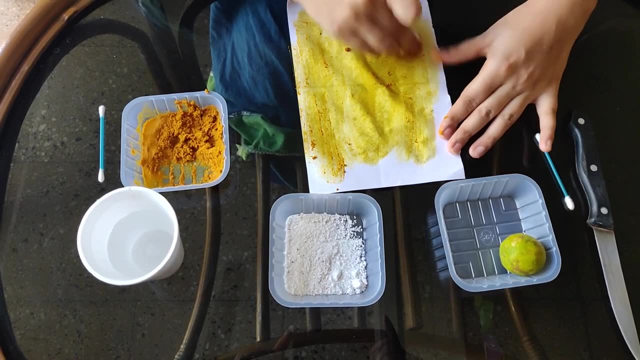 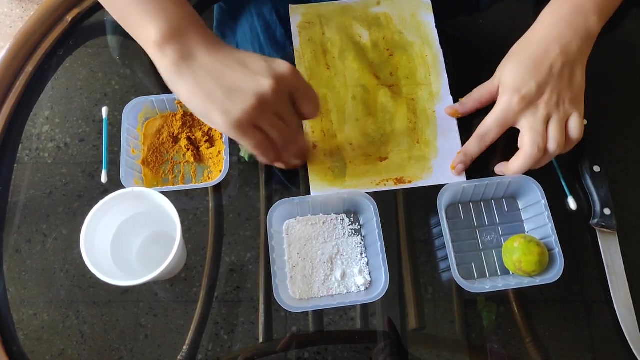 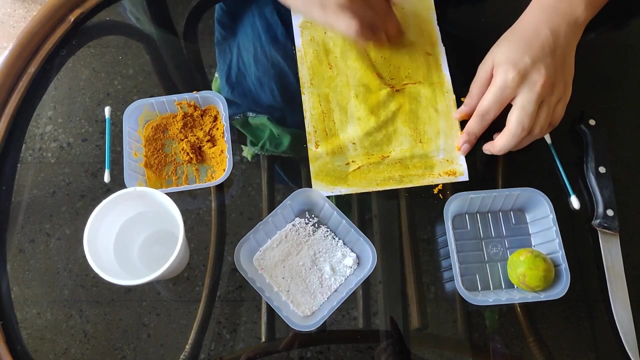 Now you can see gently I have applied turmeric paste in this paper. . See I have applied paste all over. Okay, 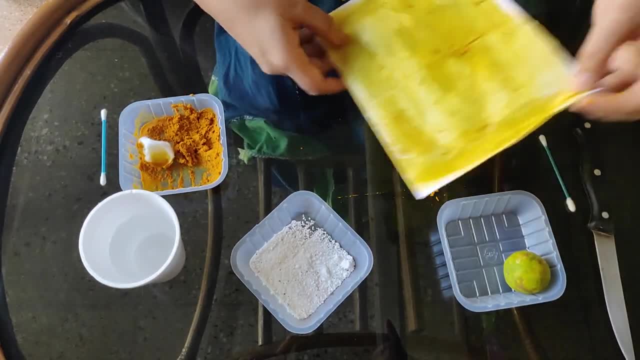 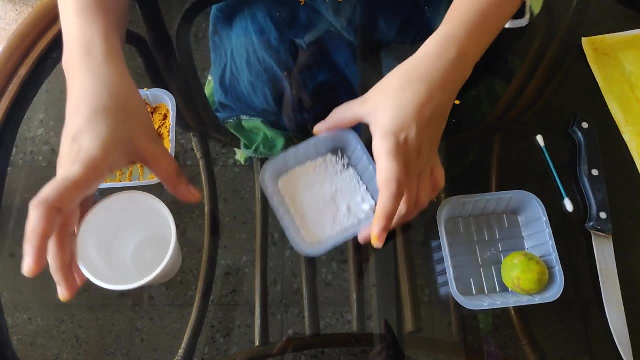 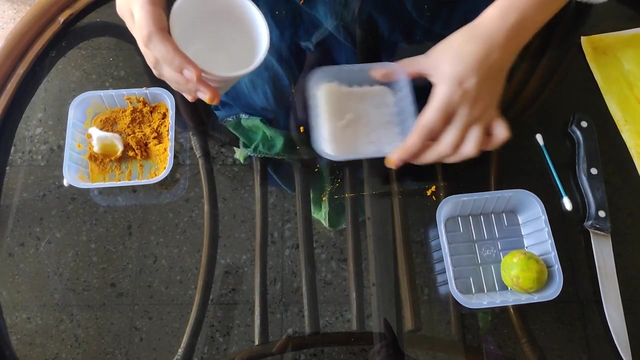 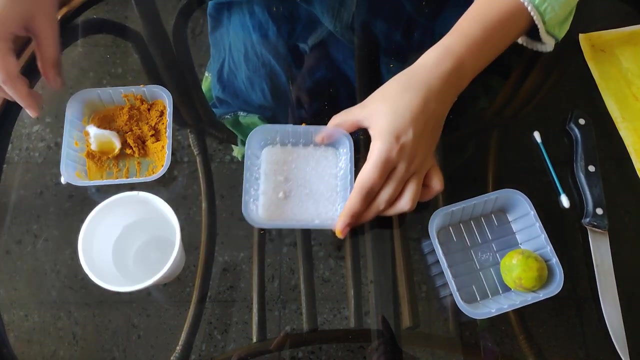 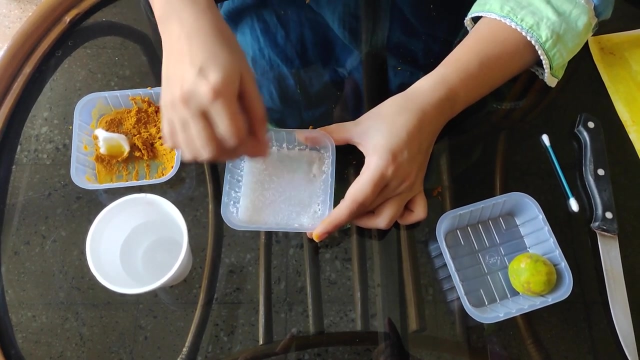 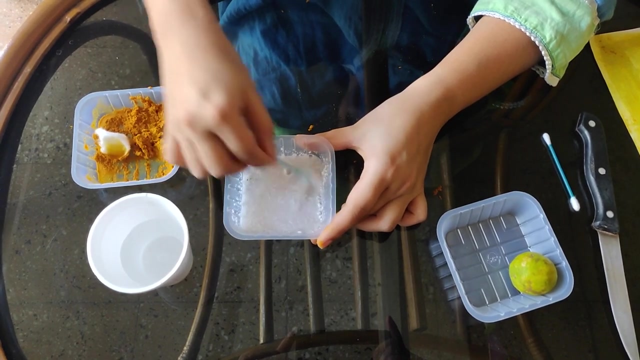 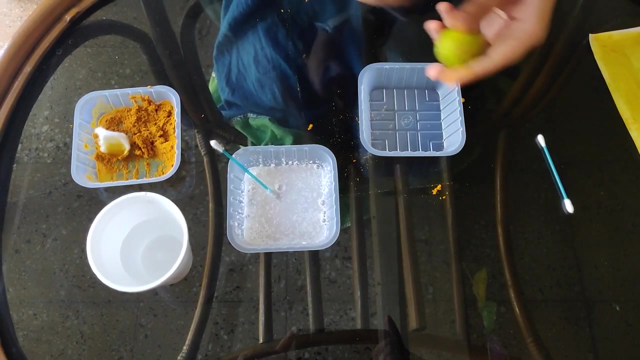 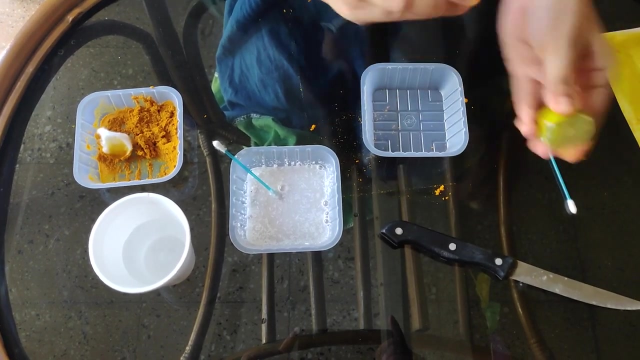 the paper and now I will allow this paper to dry for some time so let it dry for some time till that what we can do we can make our detergent solution so here it is our detergent solution this is our detergent solution that we can stir with the cotton bud because this cotton bud we will be using it afterward okay so this is our detergent solution and see this is a lemon now I will cut a slice of lemon and I will prepare its juice you can see here are 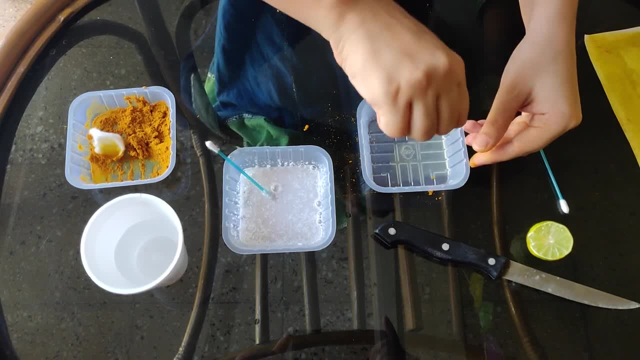 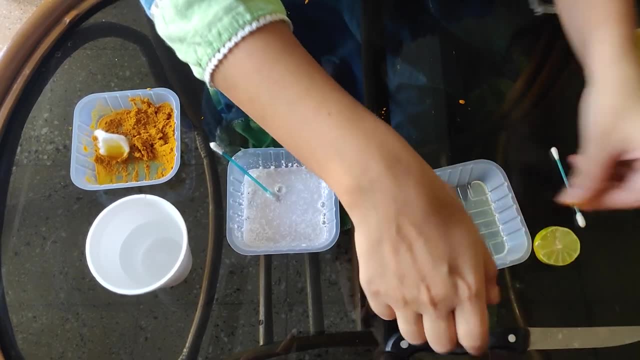 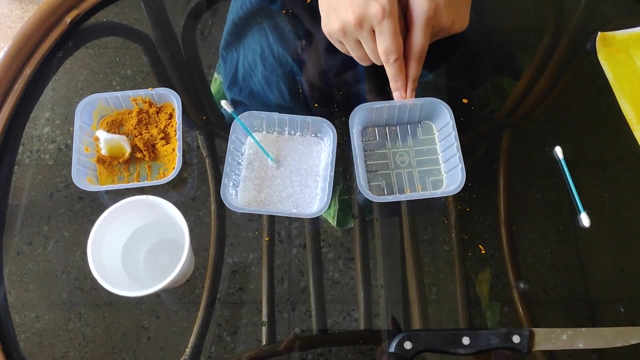 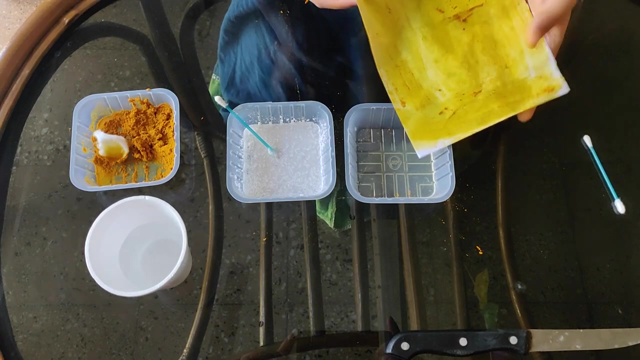 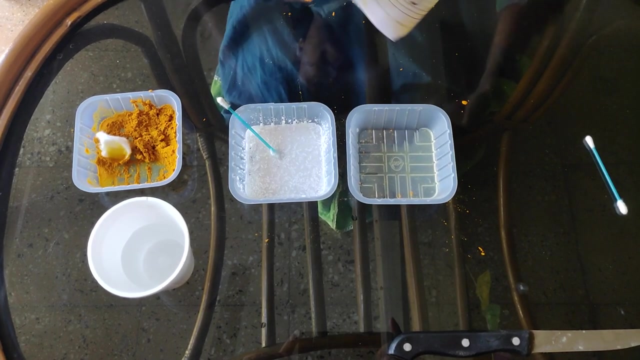 the drops of lemon okay fine so these are the drops of lemon juice now as you can see this is my detergent solution and this is my lemon juice now I will prepare this activity with the help of air but still my paper has not been dried so let it allow let it dry it for some time fine 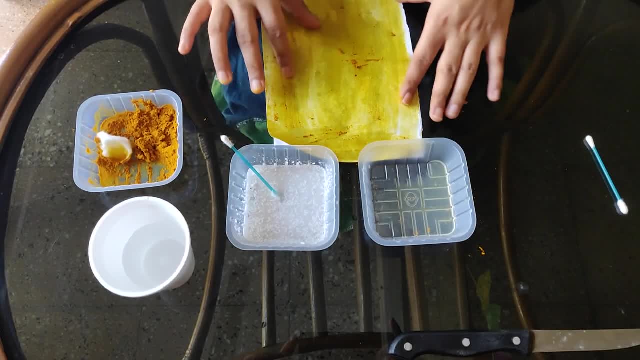 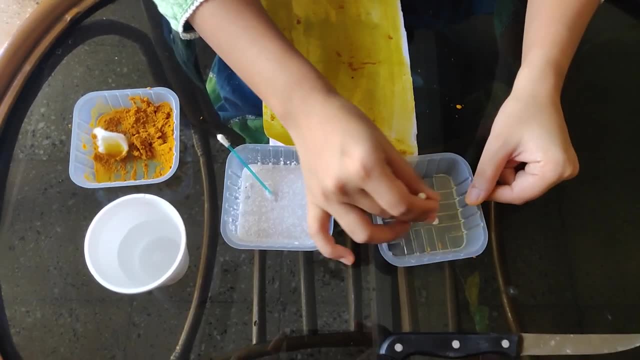 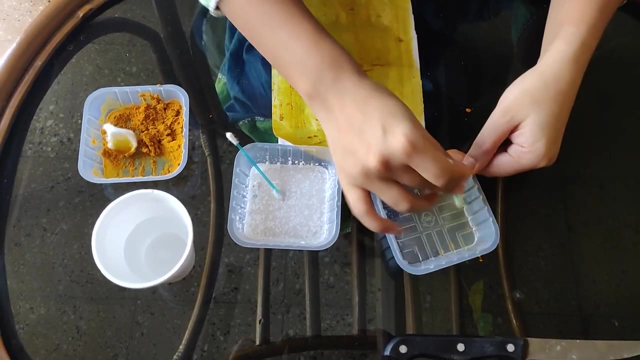 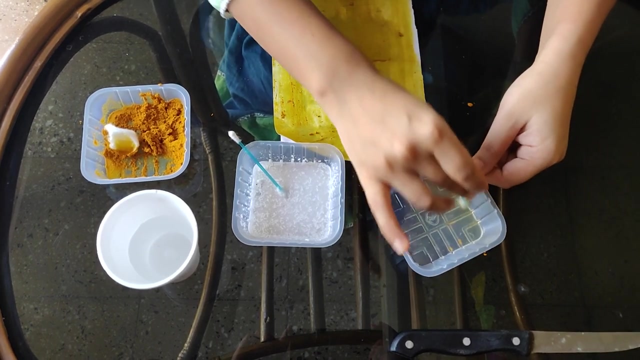 see see better now what I will do first I will test with lemon juice now you can see the effect of lemon juice in turmeric paper you can see there is lemon pick you can see the paper turns yellow as it was before yes it means turmeric 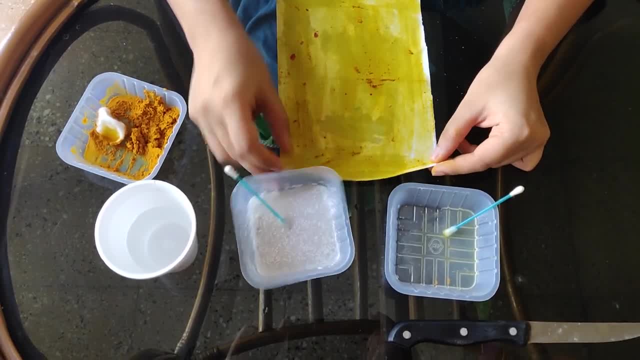 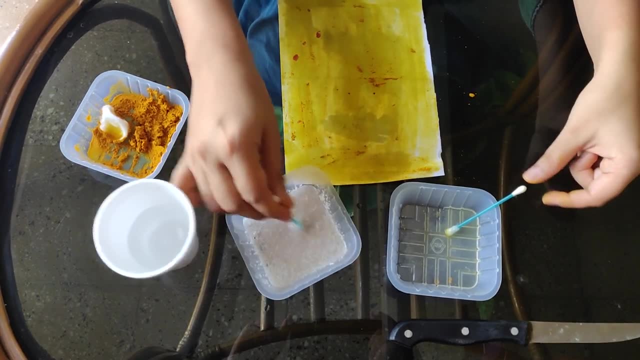 on adding acidic solution on turmeric paper it will turn yellow in color okay now let us do with the base let us do with the base what happens with the base basic solution 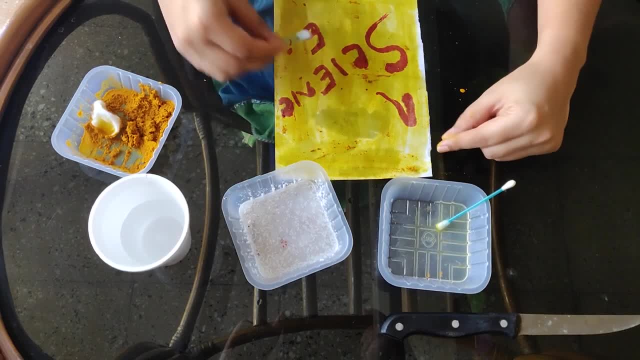 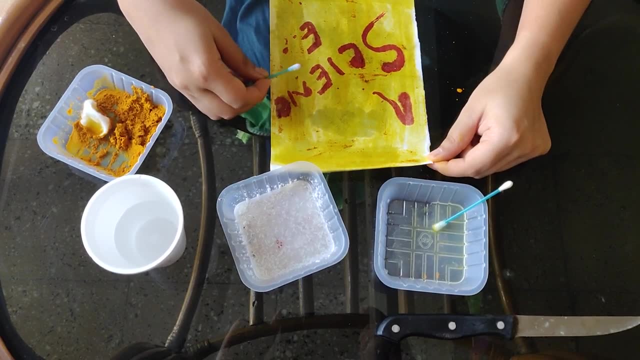 see here you can see the color change yes the color changes to reddish brown it indicates what it indicates the presence of basic it indicates the presence of basic solution okay so now